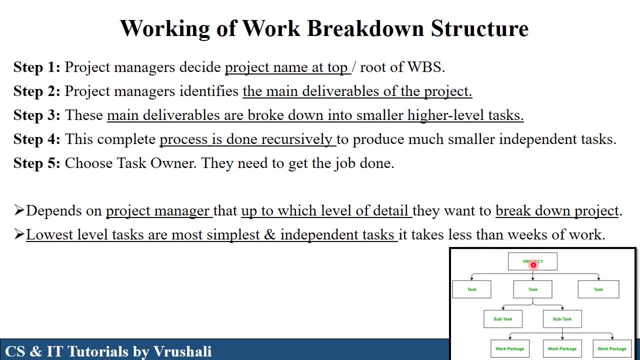 the project and this is the root node. Now, in second step project, have divided into the three main deliverable task. For example, college management system. have divided into the three main task, Like student module, teacher module and HOD module. After that, in third step. these tasks work individually in Own Night, crying day, modular system, in social area, So class management system. So class management system is organized in two multiple order of operation, as in many fields, For cities to districts, cities to Federal. 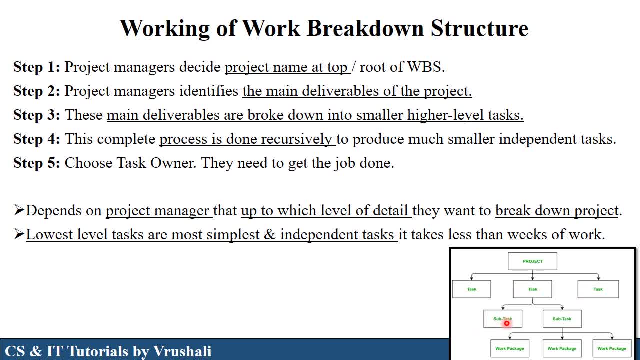 task again divided into the multiple sub tasks. for example, in student module there is a student attendance, student awards, student marks. these are the different tasks, right? so this process done recursively. generally, project manager decide that how many modules in particular project, how many tasks in particular project, then how many wbs levels in particular project. this is all decided. 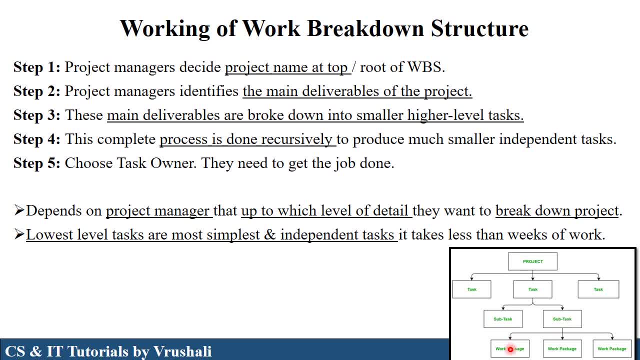 by project manager at the end. sub tasks, also divided into the different work packages. work packages is a smallest task that perform at the end of particular project. this denote the end of wbs structure. after generating wbs structure, project manager choose a task owner means they assign a particular task, a particular team lead or team member. so this is a working of wbs structure. 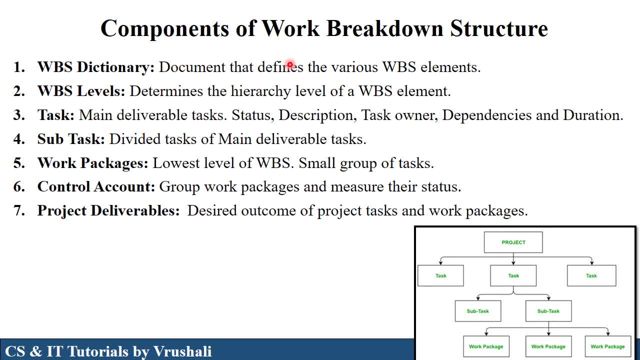 now the next topic is components of wbs. the first component is wbs dictionary. after generating this structure, this doc structure, have mentioned in particular document and this document is called as wbs dictionary. project managers send forward this document to designer and developer for development purpose. the second component, wbs level, means how many levels in wbs structure, how many. 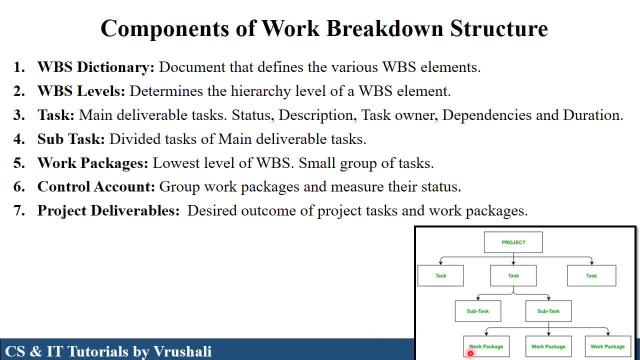 tasks. there are sub tasks, again there are sub tasks, tasks. in this way this is called as wbs levels. now the next one is a task. task means main task or main modules. sub tasks means those main tasks have divided into the different sub tasks, then work packages: work packages placed at lowest level of wbs. this is a small group of tasks which mention. 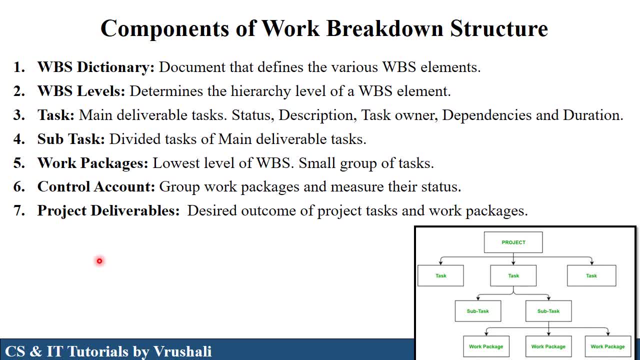 the status of your complete project. the next one is a control account. control account is a group of work packages. they measure. the status means which type of task have performed, how many time is required for completing a particular task. so basically it show the status of your particular project. 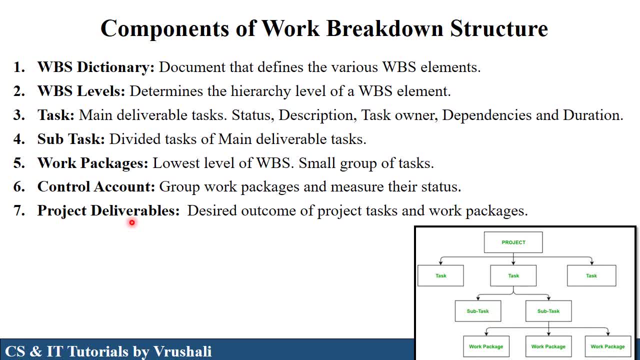 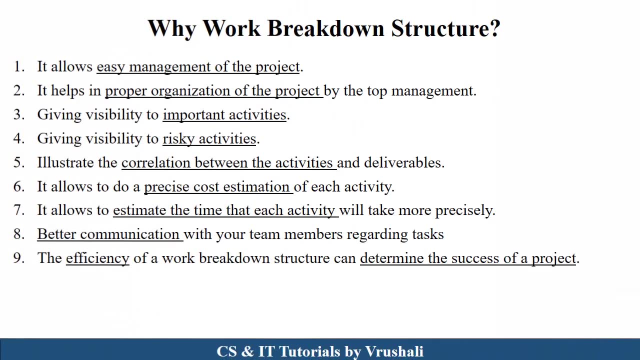 module by module. and the last one is a project deliverable. project deliver means after completing your complete project. desired outcome of project are mentioned in one task. this is called as project deliverable, which is delivered to the customer. now the next important thing is why work breakdown structure is necessary. the first thing is it allow easy management. 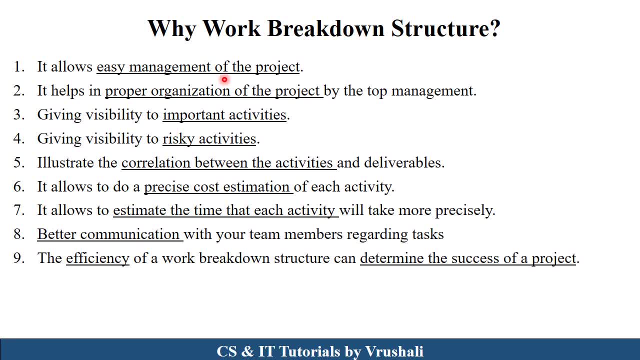 of project because they show the complete structure of project: how many tasks, how many activities and the status of your project. so it is very easy to manage. complete project and proper organization of particular project means each and every stakeholder understand the WBS structure and they understand how each and every activities have performed. so 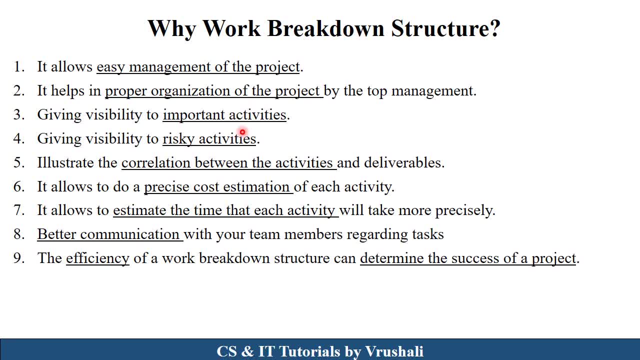 WBS structure give the visibility of important activities, risky activities and correlation between all the activities in WBS structure. it also mention the cost estimation means one task required, how many cost, and for performing 1 task how many time is required. so cost and time is also mentioned in WBS structure. so basically it provide a better communication. 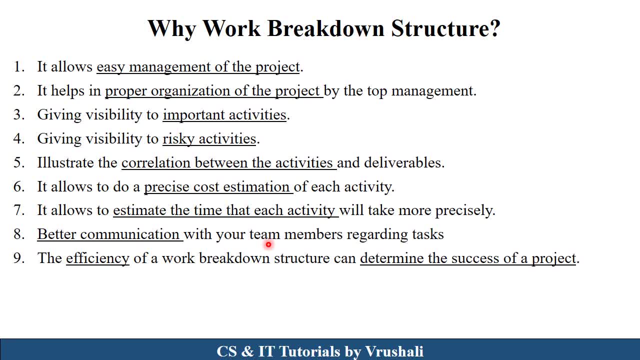 with your all team members, because this structure share with all the stakeholders. So I am going to show you how they all gather and communicate with each personnel. so what? the efficiency of WBS structure can determine success of project if you divide a complete project properly in different tasks and their subtask is. 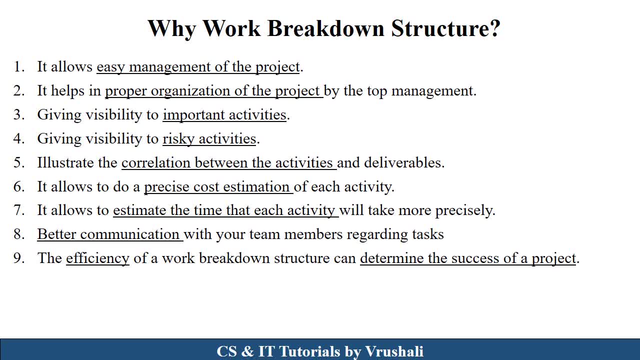 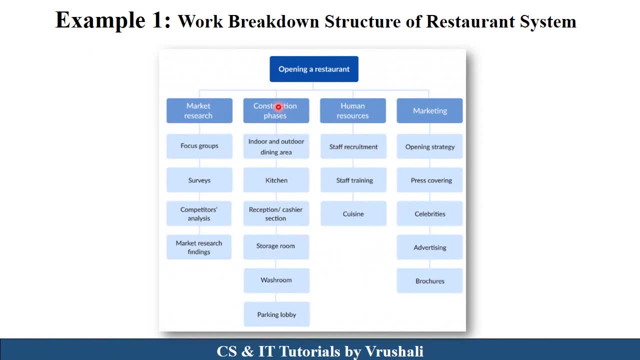 mentioned. so it is very easy to design, easy to develop that determine the success of project. now, see here these are the different examples of WBS structure. see here: this is a work breakdown structure of restaurant system. first the project name, that is, opening restaurant. then they divided into the: 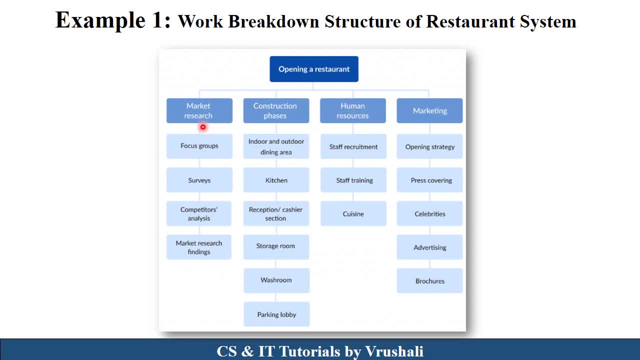 multiple tasks. the first task is market research. right first. you need to do the research before opening a restaurant. so at that time there are subtask. you can do a research by using survey. which are the competitors? are there market research, focus on group, etc. now in second task, construction phase after. 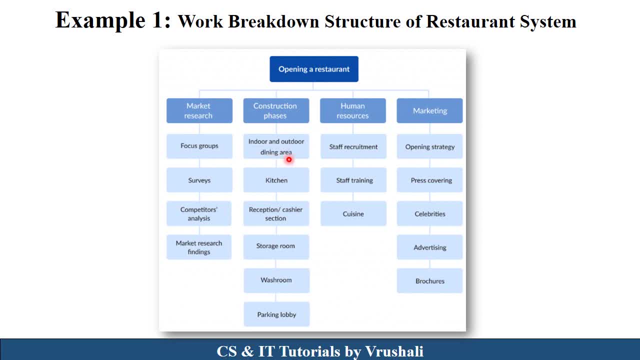 research you need to do construction of restaurant that is indoor, outdoor dining area, kitchen, reception, storage room, washroom, parking, lobby, etc. the third one is a human resources and there's subtask is staff recruitment, staff training etc. and the last one is a marketing. so in marketing you can do different activities like celebrities, advertising. 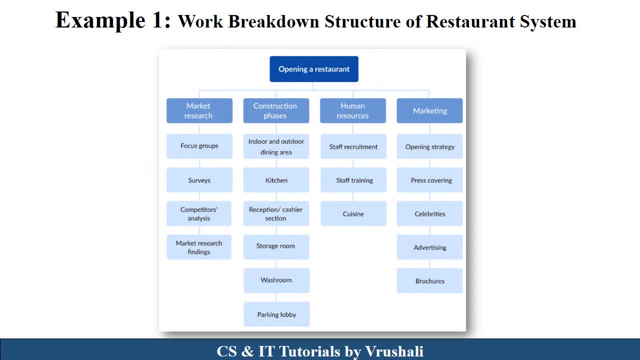 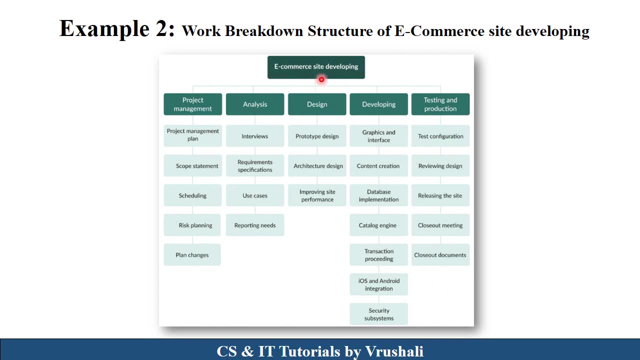 vouchers, etc. so this is a work breakdown. structure of restaurant system means it shows the proper organization of particular project and which is, which is very easy to identify, which task, which activities have performed. now the second example, which is related to e-commerce site developing. see here this is a WBS. 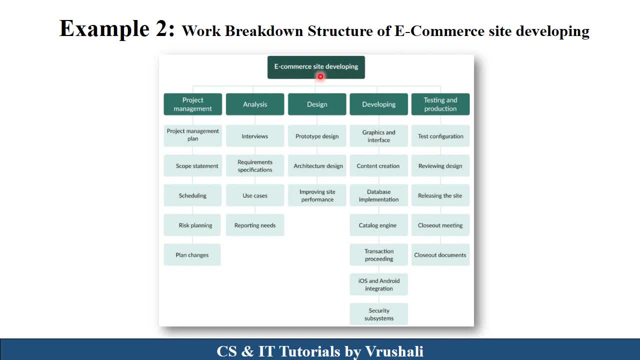 structure which is related to e-commerce site development. see here this is a WBS structure of actual development. here this is a project name and it can be divided into the multiple tasks. the first task is project management in software development lifecycle. first you need to manage a plan, scope statement, scheduling. 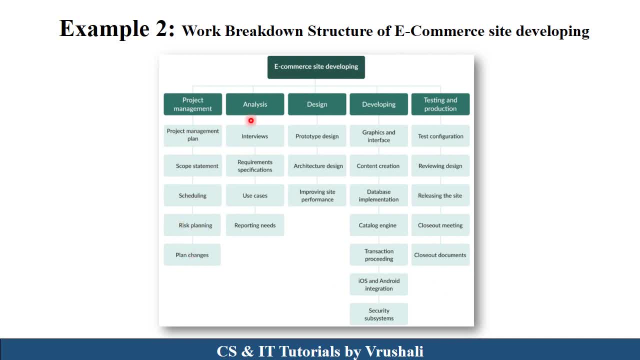 risk of planning, etc. then second one is a analysis. you can do a analysis by requirement gathering, interview, use cases. the third one is a design in design. the subtask are prototype design, architectural design. after design there is a developing, that is, graphics and interface developed, database implementation etc. and 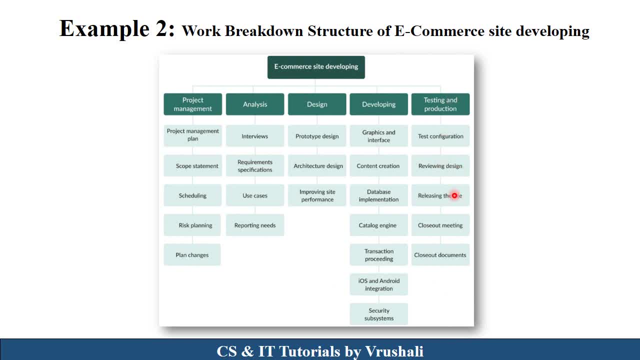 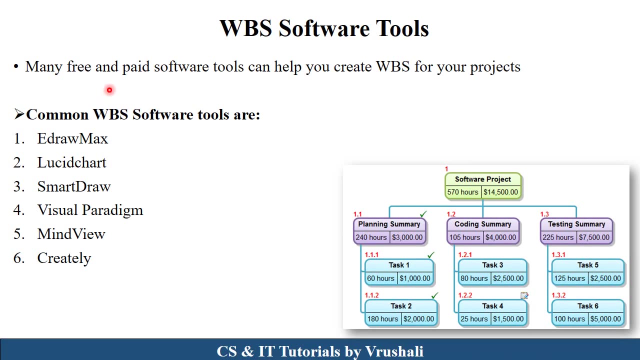 last one is a testing and production here: reviewing design, releasing site, close out meeting, close out documents, etc. so basically it shows the complete structure of project in sequential manner. so this is a WBS structure. now in market there are some free and paid software tools are available for creating this work: breakdown structure tools like e-drawmax. 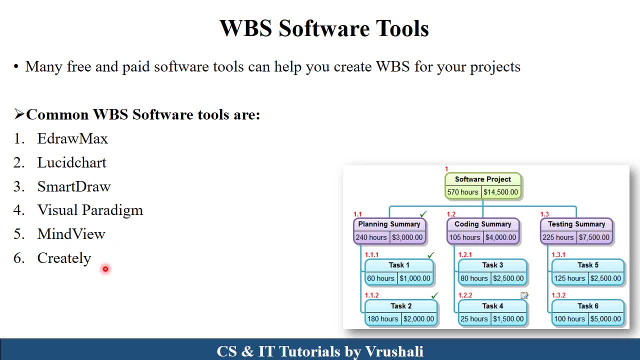 lucid chart, smart, draw, visual, paradigm, mind, view and creatively. you can use any particular software for creating this WBS structure. see here in this diagram, here there is a software project. these are the different tasks and these are the different tasks. so for completing a planning, the required 240 hours and the particular cost means it also mention how. 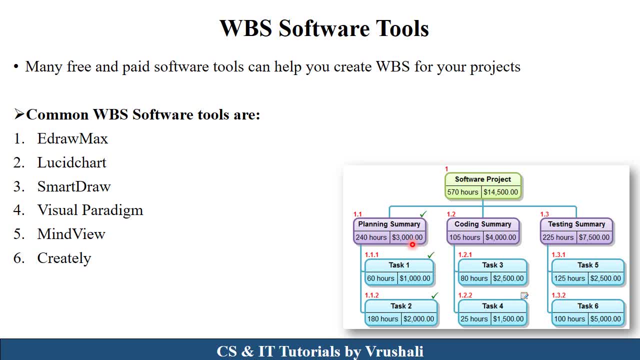 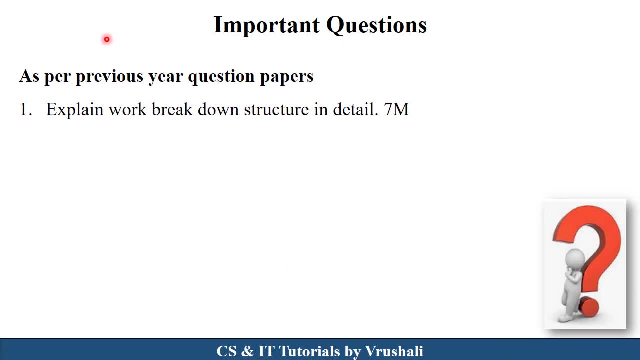 many time is required for completing a particular activity and how many cost is also required. so this is a complete structure of WBS. As per your previous year question paper, this is one of the most important question, like explain work breakdown structure in detail. here you have to explain the theory plus example. 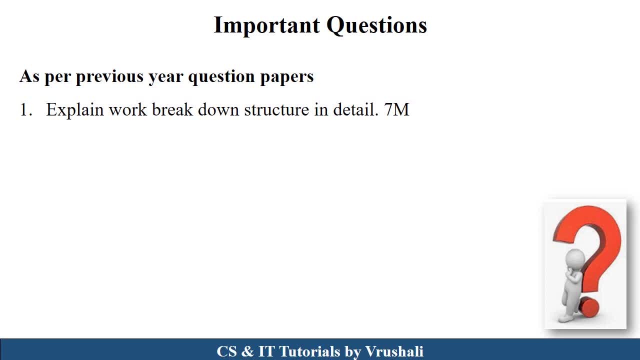 you can take any example for explanation with diagram for 7 marks. this is all about WBS. thank you, keep learning.